The only naturally occurring isotopes of uranium are U-234,, U-235, and U-238.. And of those naturally occurring isotopes, 99.3% of all that naturally occurring uranium is U-238.. Only a very small fraction, 0.7%, is U-235.. 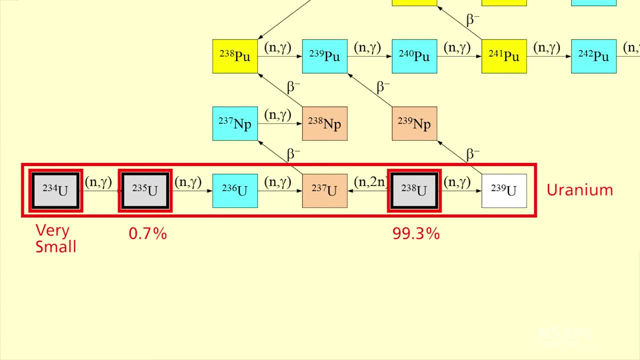 And there's a very small fraction of U-234, much less than that Of those isotopes. when we want to use this in a nuclear reactor, we would like to enrich in the isotope U-235.. Typically, power reactors would enrich the naturally occurring material from 0.7% to somewhere around 3% to 5% U-235.. 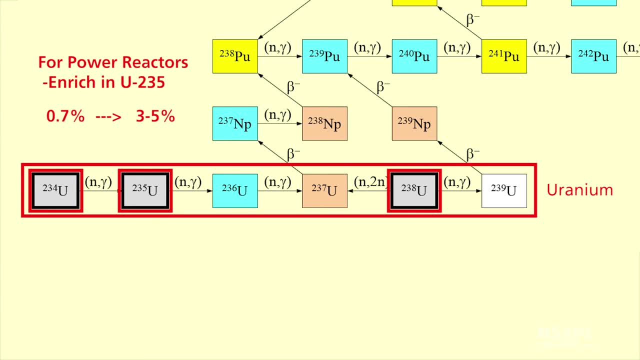 And this material, then this U-235, is what then would cause fissions inside of the reactor and give you power. So most of the reactions then that would occur in the U-235 isotope, for instance, would be fission reactions. 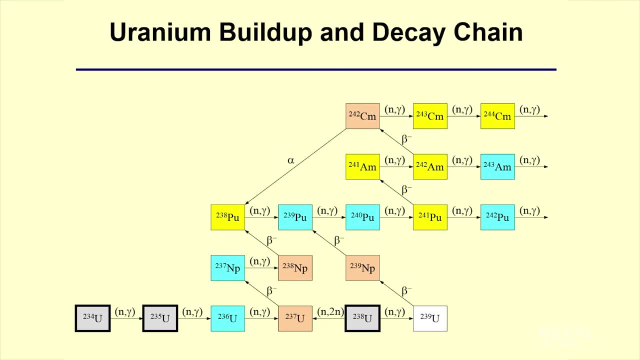 However, on occasion when irradiated in a reactor, some of the neutrons will get absorbed in what we call a radiative capture reaction, which is a reaction then that would lead to the production of, let's say, the isotope U-236.. 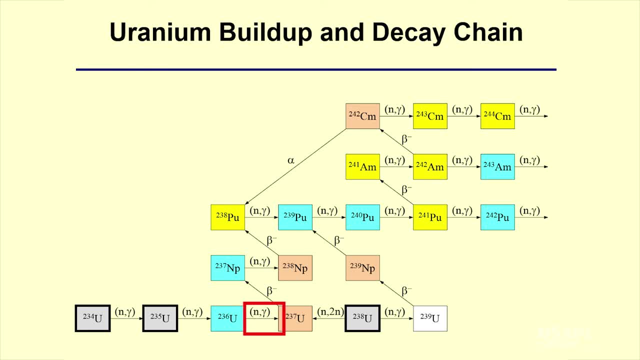 That U-236 could also absorb a neutron and produce U-237.. U-237 then could beta decay, which is releasing an electron to produce neptunium-237.. Neptunium-237 is a different element than uranium. 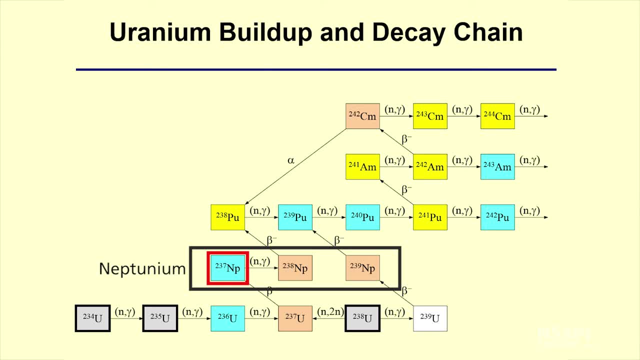 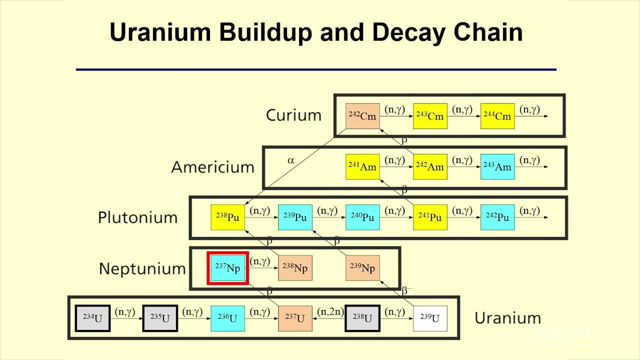 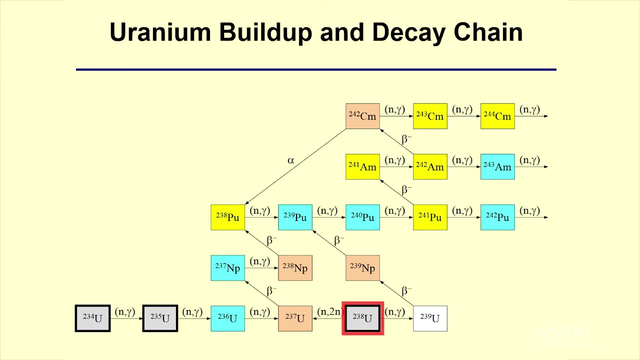 Neptunium-237 is of the element neptunium, and so each of the rows on this chart are individual elements, So the element of uranium, neptunium, plutonium, americium and then curium. As we irradiate this material, U-238,, for instance, would absorb a neutron and produce U-239.. 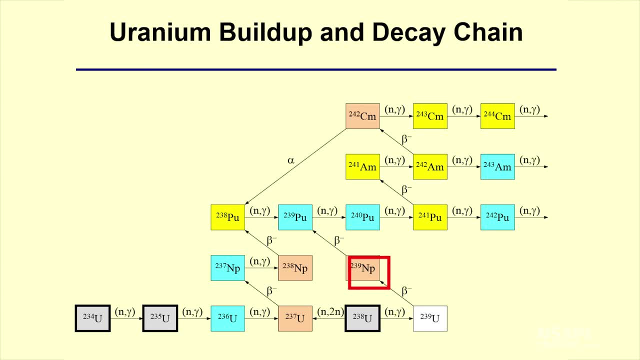 U-239 then would go through two subsequent beta decays to plutonium-239.. Plutonium-239, then, is the material that's principally used in most nuclear weapons. Plutonium-239,, if it continues to be irradiated in a reactor, would produce the higher mass plutonium isotopes of plutonium-240,, plutonium-241, and plutonium-242.. 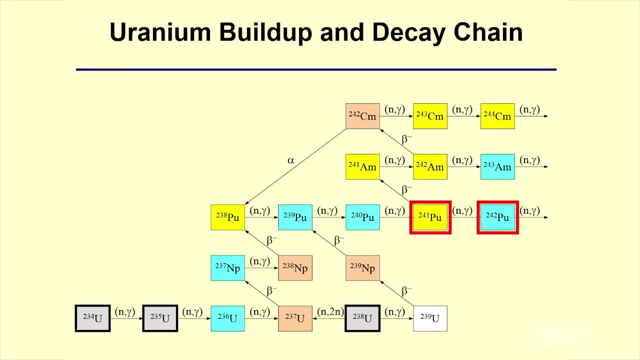 And of those isotopes, plutonium-241,, for instance, could beta decay to americium-241, which could continue the chain. So as we continue to irradiate a fuel in a reactor, we would expect to see some of these other isotopes get produced. 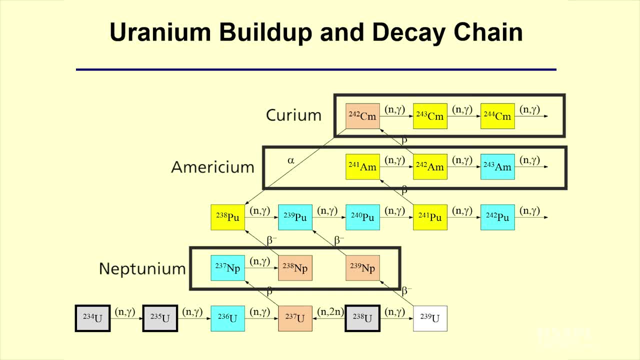 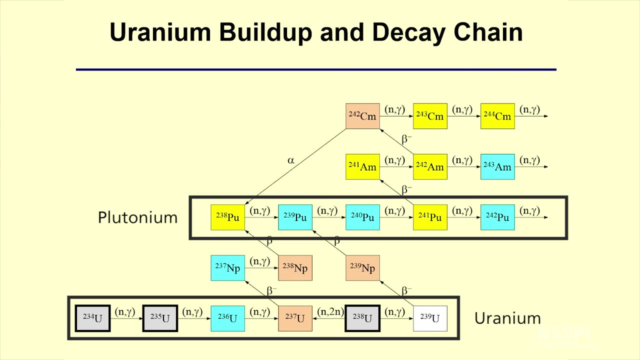 The elements neptunium, americium, curium and so forth are elements that we refer to as minor actinides. They're small players inside of the reactor, in that they are small absorbers, things like that. The principal elements of interest to us are uranium and plutonium, both of which can serve as fuel sources inside the reactor. Thank you.